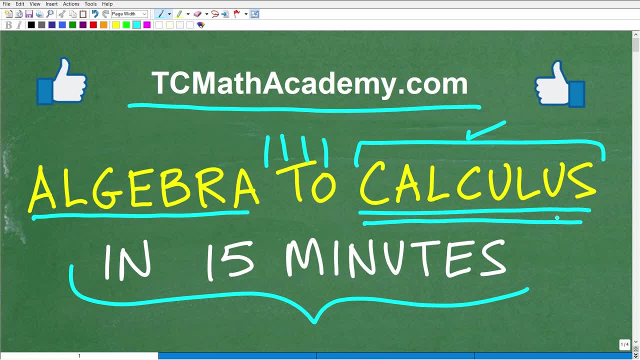 calculus if it interests you, as calculus is an awesome, awesome mathematics and it's quite different than algebra. But in order to fully understand calculus, you're going to have to get through all these other courses which we're going to be talking about here in just one second. Also, if you need math help with the course you're taking, test prep or homeschooling, make sure to check out my math help program at TC math academycom. You can find a link to that in the description below. Matter of fact, I'm going to leave a link to all my 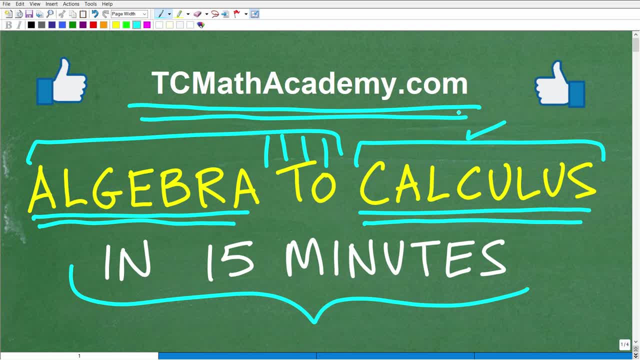 math courses, my main math courses, which would include algebra, geometry, algebra two and pre calculus and pre algebra- for those of you out there that need to take that course. And obviously pre algebra would be the course that you would take before algebra or algebra one. And if this video helps you out, don't forget to like and subscribe, as that definitely helps me out. Okay, so I've got about 15 minutes and all I want to do is just give you some general 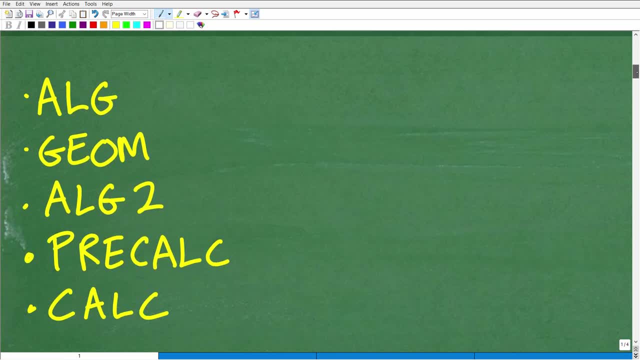 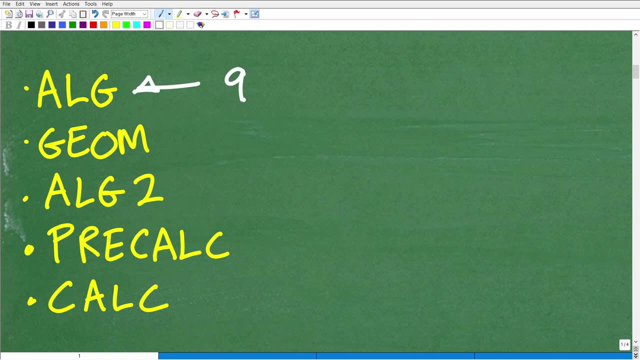 sense. For those of you out there that are, you know, wondering: hey, what math do you have to take in order to start from algebra? and algebra or algebra one is the most kind of typical math course that students would take, let's say, at the ninth grade, high school level, right? So then they would move on And generally- I'm speaking in generality, but this is most people's track here- So as a freshman in high school, you start off in algebra or algebra one, then 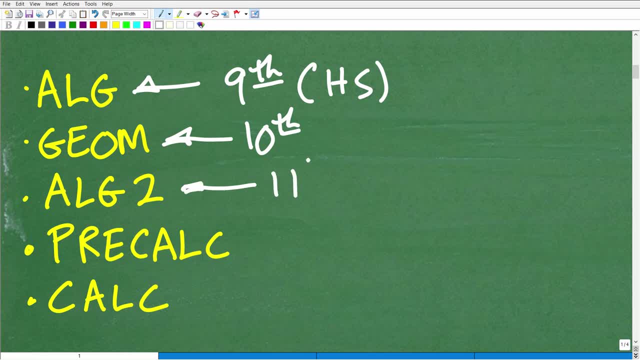 as a sophomore, 10th grade, you move on to geometry. then in the 11th grade you would take algebra two And then for those students that really want to, you know, get ready for college level mathematics, you can opt in to like a pre calculus course. there's other options for most students. Now I will say this: the majority of high school students have to at least get through these courses here: algebra, geometry, algebra two- okay, even if you're not going to college. 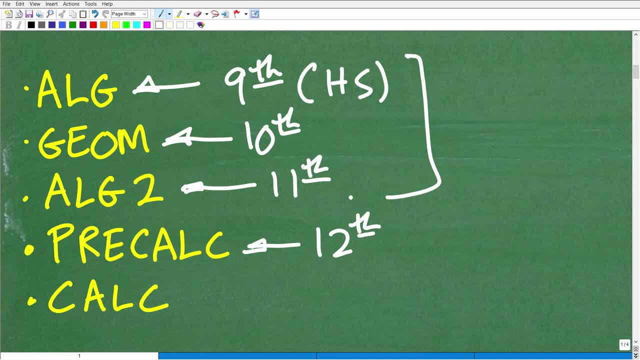 generally speaking, all right. so this is a pretty typical track for almost all students. Pre calculus is only going to really be there for those students are definitely going to college. there's other math that you could take, or maybe you don't even have to take a math class- maybe business math, consumer math, statistics, whatnot- But if you're looking to take calculus, you want to take pre calculus, right. This is definitely a challenging course, And then you would move on finally to 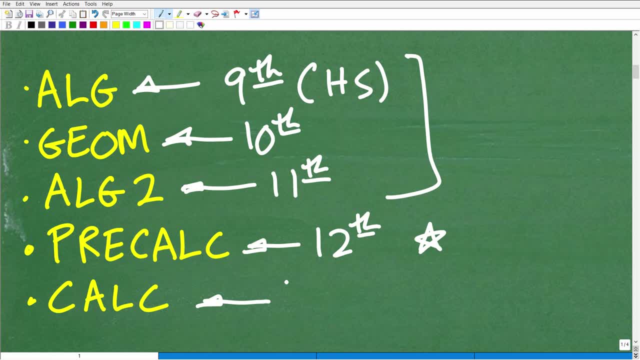 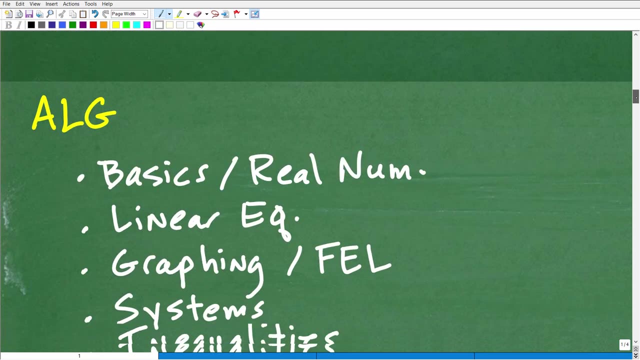 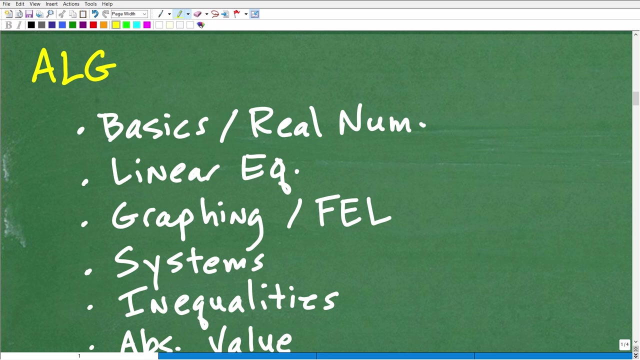 calculus is a freshman in college. this is a very typical kind of track. So these are the courses here that we're going to look at and just take a quick peek at what you learn in each of these, right, And I'm talking about a very fast overview. So let's go ahead and talk about algebra. So what do you learn in a basic algebra- algebra one course. Well, let's just kind of go through some main concepts here, All right? So first of all, you're going to be reviewing all the basics. 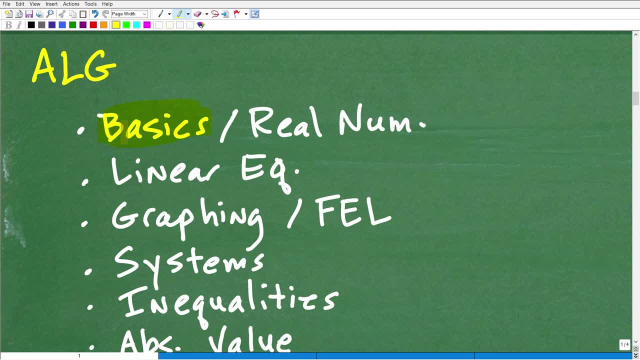 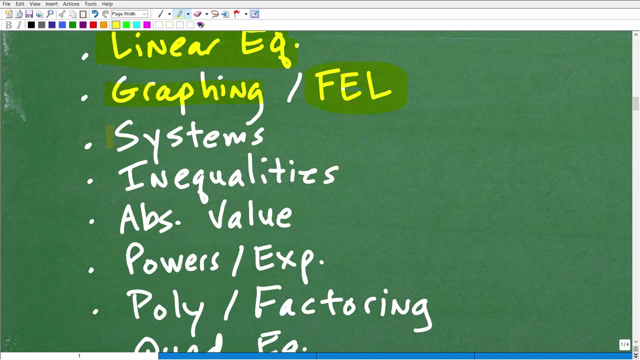 stuff like what's a variable, the order of operations, all that kind of stuff from middle school and pre algebra. real numbers, ie positive and negative numbers. you definitely have to know how to solve equations, what we call linear equations. you got to know how to graph lines. you got to know how to find the equation of lines, systems of linear equations. by the way, anything I mentioned here, if you have you don't really know, or if you're struggling with check out my respective courses, Just follow the links in the description. Also, I have a ton of 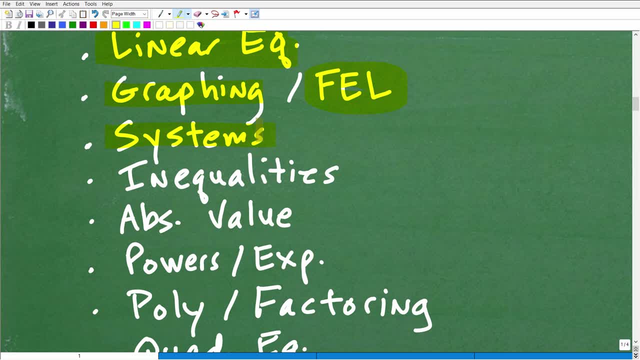 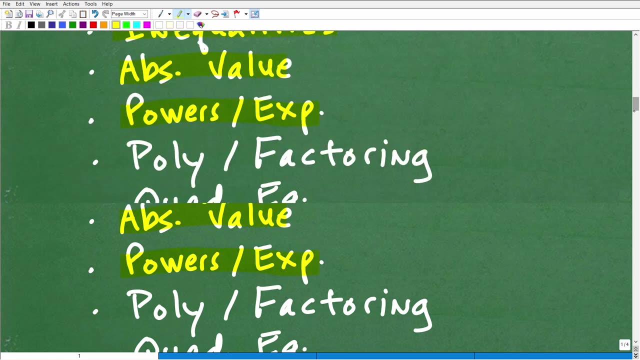 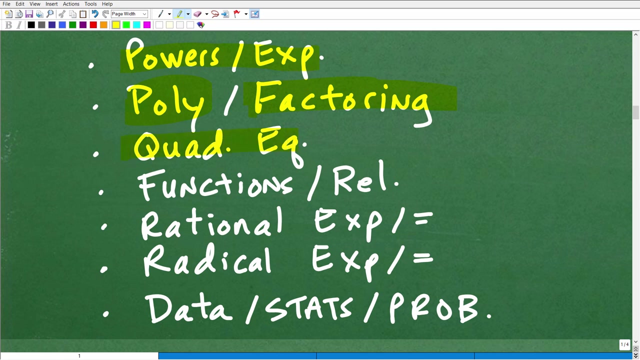 additional videos on all these topics on my YouTube channel. Okay, but we're just kind of highlighting the main kind of chapters in these courses. Let's go ahead and continue on Inequalities. okay, you need to learn this in algebra: one absolute value. inequalities, equations, powers and exponents. you can see it's quite a bit of material. polynomials: how to add polynomials, subtract, multiply, factoring polynomials, quadratic equations, quadratic formula, functions, relations domain. 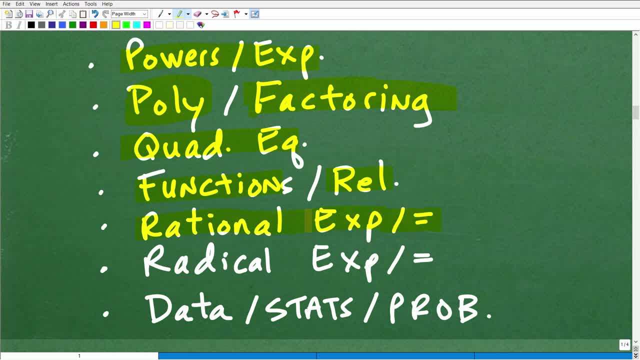 range. then you got rational expressions and equations, which is a pretty big deal right here, got to learn how to find the lowest common denominator of rational functions, which is not exactly that easy. Well, it's not overly difficult, but it tends to confuse a lot of students. Then you get into radical equations, expressions and equations and extraneous roots, And then then you have, generally speaking, in most algebra courses a data component. right, you're going to learn about frequency charts and 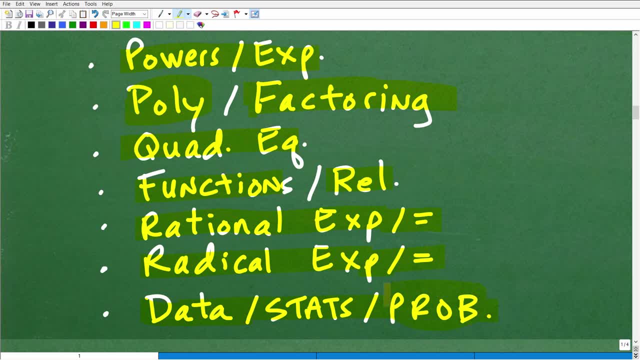 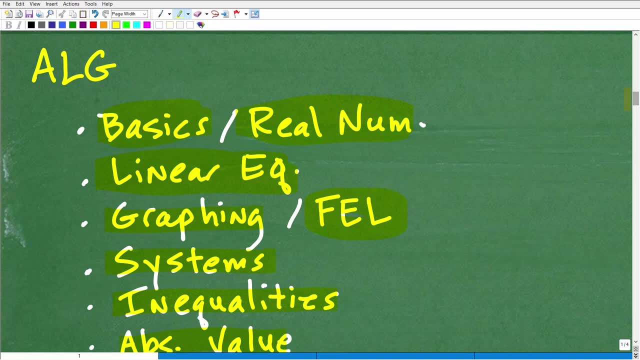 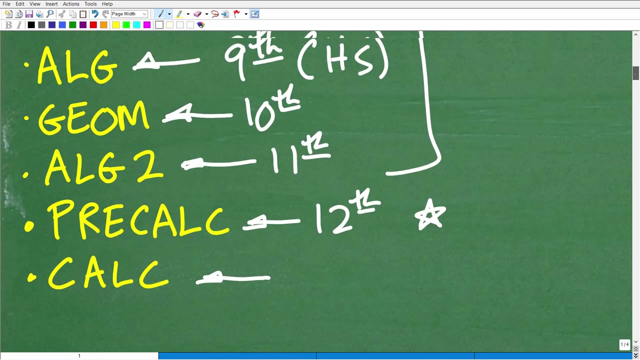 averages mean median mode and basic probability and counting theory. So this is quite a bit of stuff you have to learn in algebra one And what you know. I've taught all these courses for decades. what I've tend to found out, or tend to see, is that how you do an algebra one is going to affect- you know- pretty much the rest of how it's going to go for your high school, you know, or your prerequisites to get to calculus. Okay so 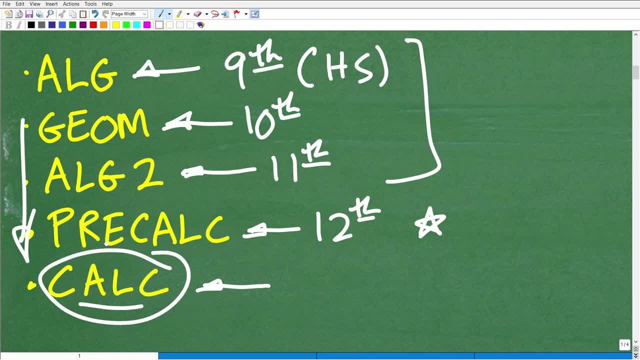 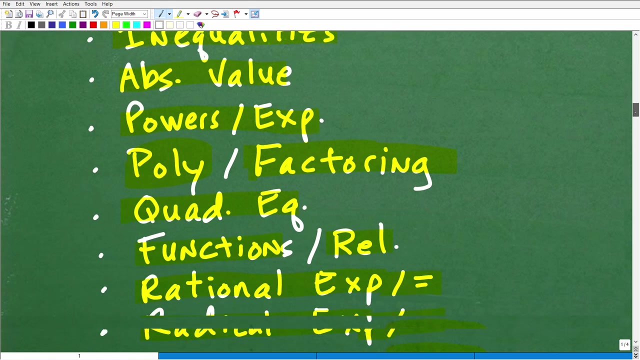 if you're struggling. let's suppose you're taking pre calculus or calculus. you're having a tough time. there's a good chance that maybe you didn't do as well in algebra one as you, you know, should have done right, And there's a lot of reasons for it. Maybe you were distracted. Maybe, you know, you didn't understand your teacher. But I'm telling you right now: algebra one is an absolutely critical course to master because it really lays the foundations for all you know, the rest of the mathematics you're going to have to learn Now. let's move into geometry Now, high school. 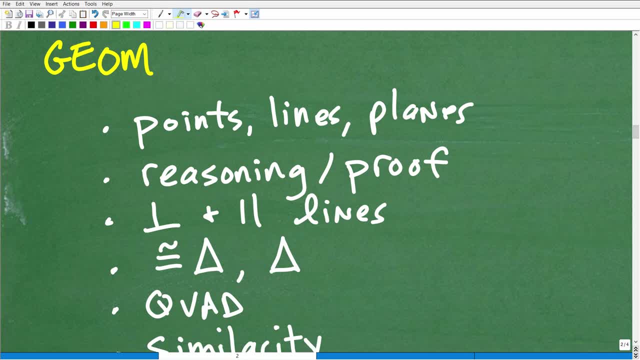 level geometry is far you know. when I say geometry, a lot of students are like: Oh, you're going to find the area and volume and triangles. Well, high school level geometry is a lot more than that. Okay, do learn a lot And you have to, you know, really get your geometry down at, you know, when you take a high school level geometry course, because you're not going to see these topics again until you. you know, get until, let's say, more advanced math in college. But let's just do a quick overview, right? So in geometry you're going to be learning a lot about points. 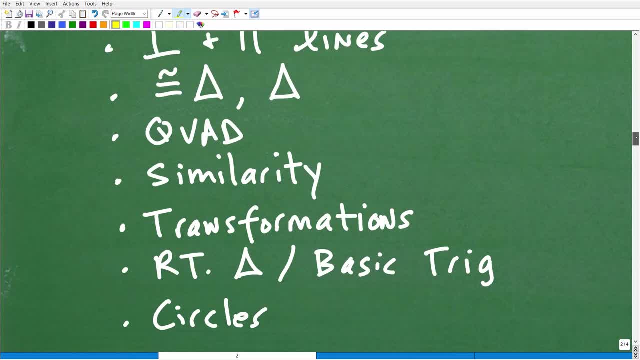 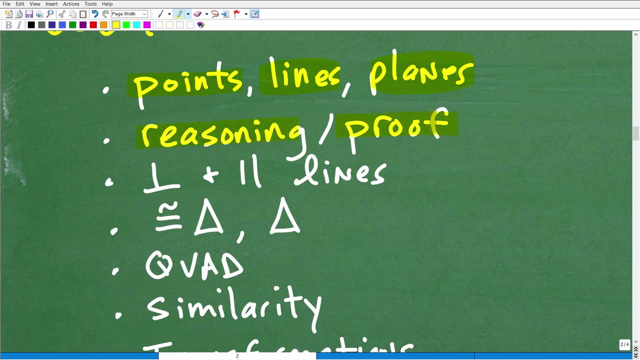 lines, planes, all the notations and properties that go with that. okay, which is a lot Reasoning and proof. that's a big thing in geometry, deductive reasoning, logic, you know what's a postulate, what's a theorem, How do you create or write a geometric proof? Another thing is: this is a generally like a chapter in and of itself is perpendicular and parallel lines: Okay, all the properties and 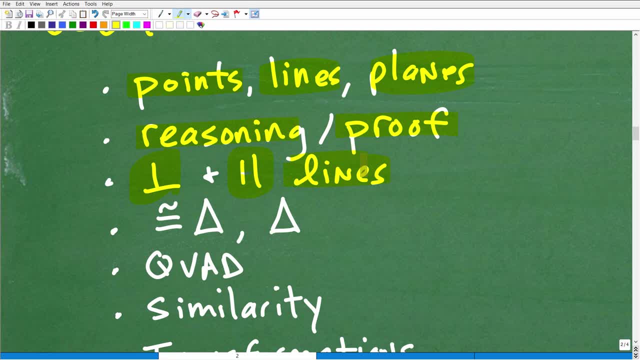 theorems and postulates. they're transversals, alternate interior angles, all this stuff. Again, if you don't know what I'm talking about, you will learn this. Or if you want to learn it, you can take my course or another course. But again, this is what you're going to have to learn in high school level: geometry. Then you have congruent triangles and a lot about triangles and geometry, And you would. you know. you know a triangle is just one shape, But you know you might say: well, why don't we just obsess over triangles? What triangles are? 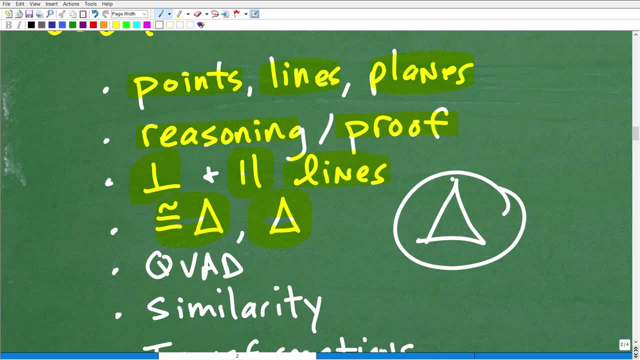 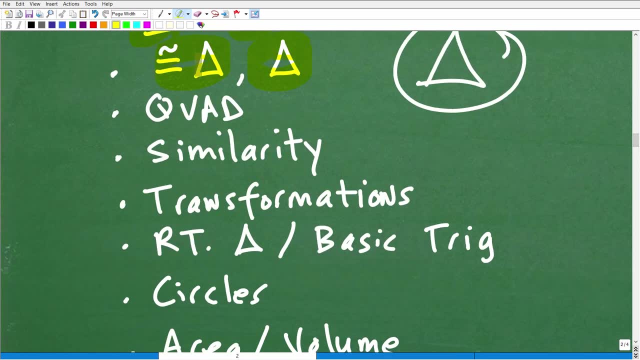 extremely important And you're going to learn a lot about the properties of triangles: congruent triangles, similar triangles- a lot to learn about triangles, Okay. so another topic you're going to get into is quadrilaterals and polygons. Okay, so that's a four sided polygon And there's all. 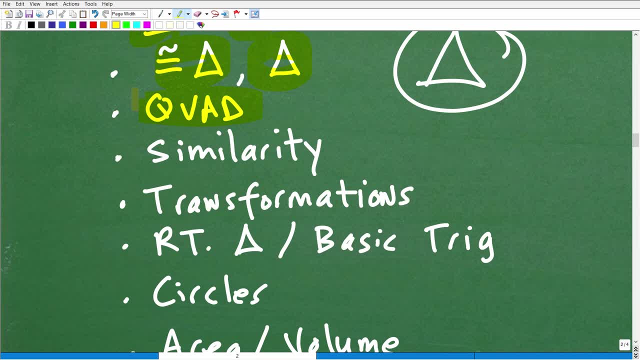 different types: trapezoid, rhombus, etc. etc. Probably heard some of these terms. then you're going to get into similarity. Okay, and that's another big topic that you're going to have to master: Transformations. that has to deal with rotations, dilations, reflections, right. So if 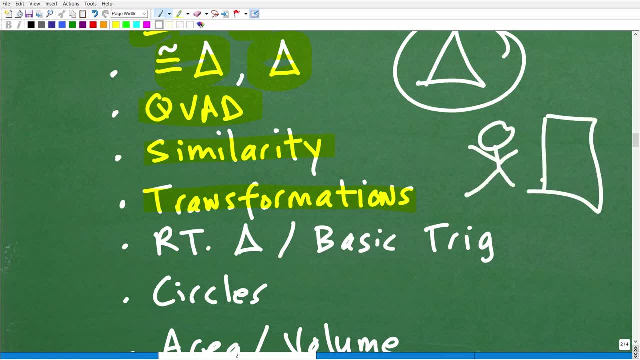 you see yourself, you know, in the mirror right you're looking at a reflection of yourself. And if you kind of like, you know, take an object and rotate it 90 degrees, what does that object look like? This is what we call transformations. Okay, and there's a few different types. And then 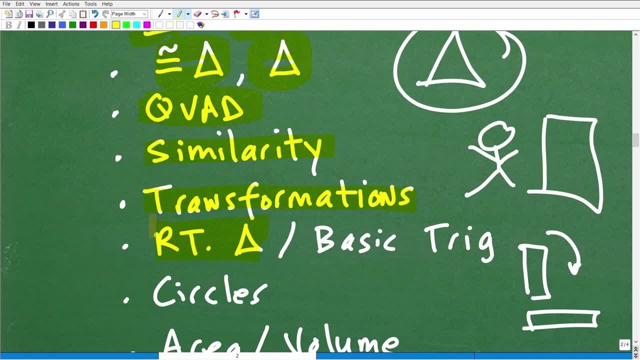 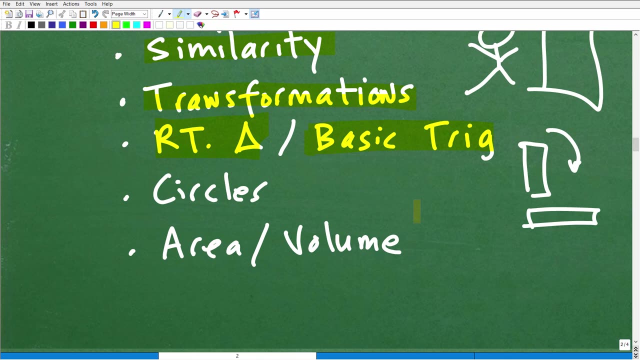 you're going to get into more stuff about triangles, to include right triangles, special right triangles, which is kind of leads you into basic trigonometry. So you really have an introduction to trigonometry in geometry. Okay. so like things like sine cosine, tangent, of course, 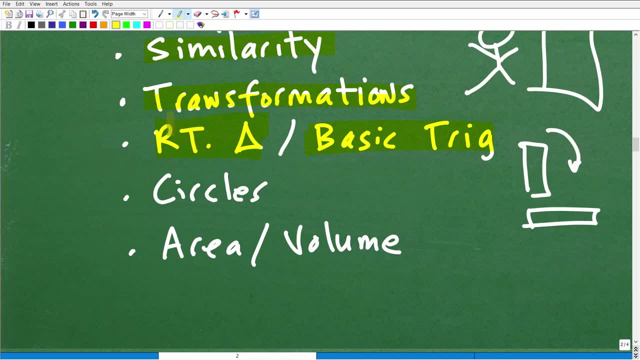 right triangles, you're going to learn about the Pythagorean theorem: a squared plus b squared is equal to c squared, etc. So if you're kind of flabbergasted right now, hey, listen, you know this is a full year. 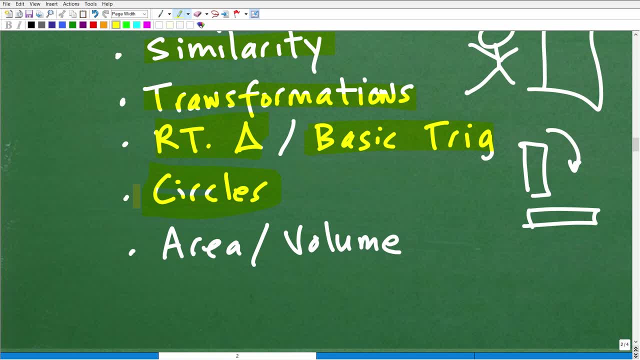 course and a lot to cover. Let's go ahead and continue on. You're gonna learn a lot about circles. okay, much more than just finding the area or circumference. you're gonna learn about arcs, chords, inscribed angles. there's a lot you need to know about circles. And then finally, 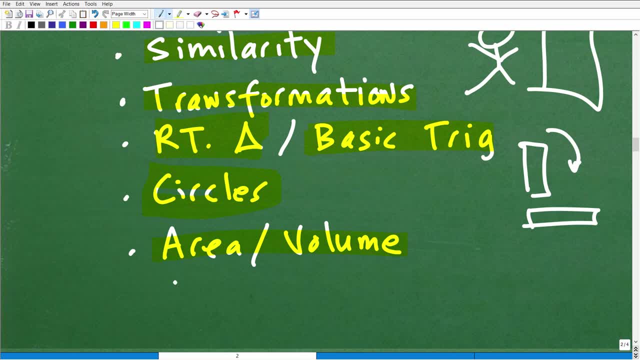 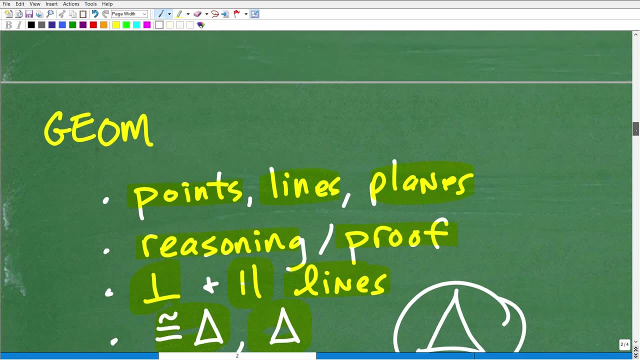 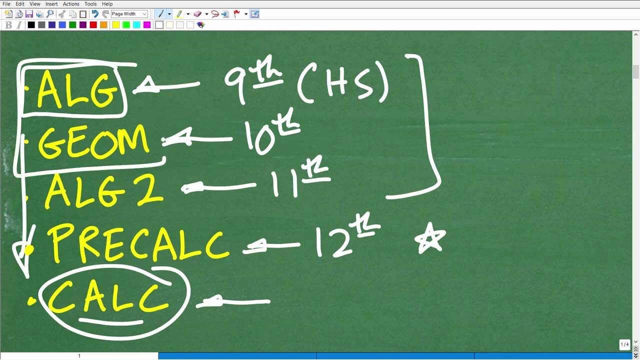 you do get into area and volume and sector, area, arc length, all this kind of good stuff, So you know lots to learn in geometry. Okay, so typically most students are going to take algebra one and geometry, in this order. let's take a look at this right here. you would want to take? 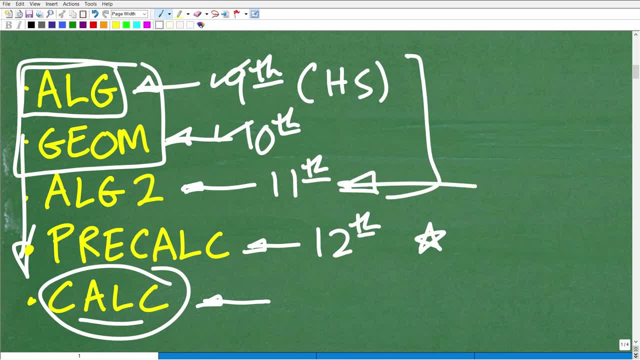 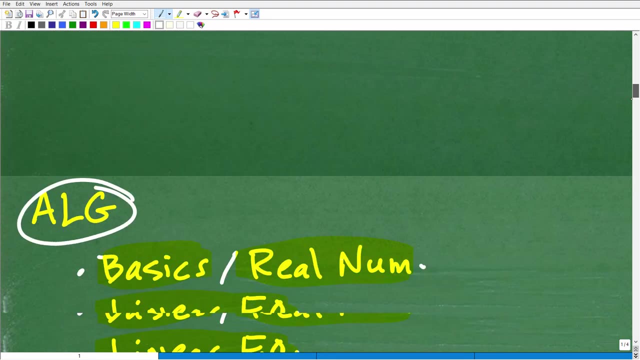 these courses in this order because in your 11th grade year you want to have these courses done So you can be ready for tests like the SAT and ACT, which is typically like 5050 in terms of the algebra and geometry, or maybe like 6040, a little bit more algebra than geometry on those exams. 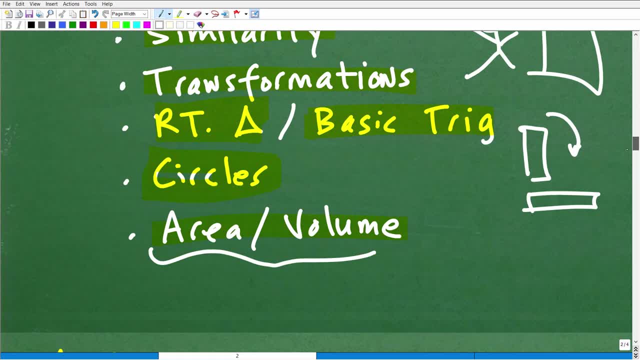 where you want to get those out of the way, And you can see it's a lot. Okay, so let's go ahead and take a look at Algebra two. Well, in Algebra two, you're pretty much going to be doing a review of 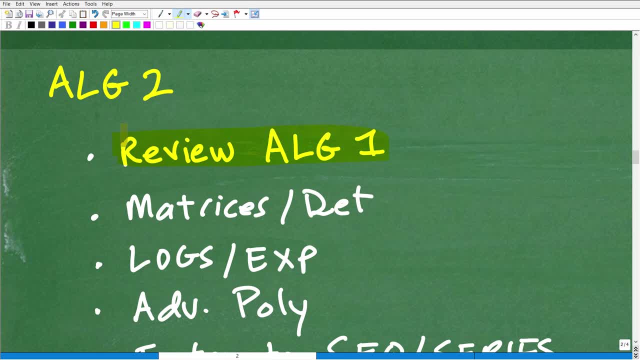 Algebra one. it's like everything in Algebra one, which we saw is a lot you're going to be kind of doing again, okay, so you know it's, it's just more of the same, if you will, but then you're. 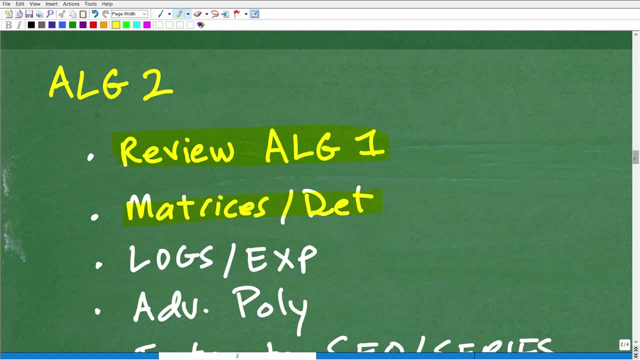 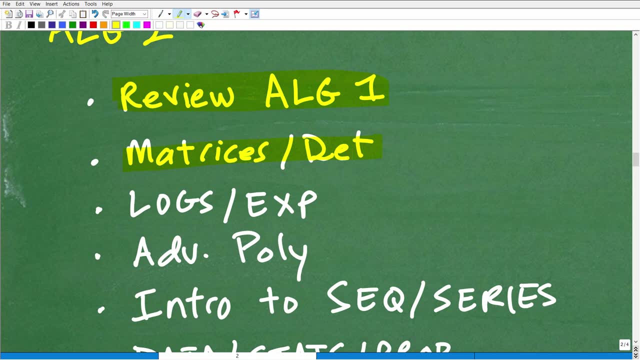 going to be introduced to new, more advanced algebra topics, things like matrices, determinants again. if you don't know what these things are, you'll certainly learn them. Another big thing that's generally taught in most Algebra two courses is logarithms, which are part. 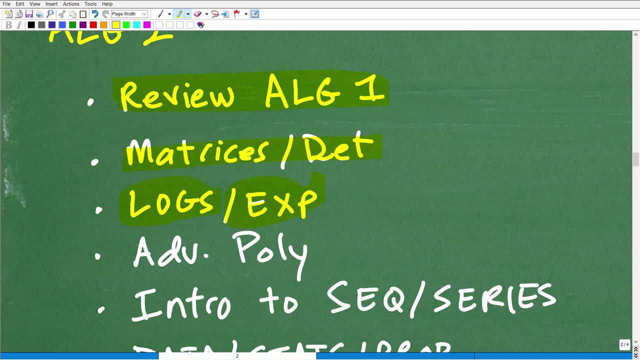 of like exponential functions. that's generally like one chapter. then you start learning about advanced polynomial theorems, how to solve higher order polynomial equations. So in Algebra one you solve things that are like quadratic equations, right second degree polynomials. 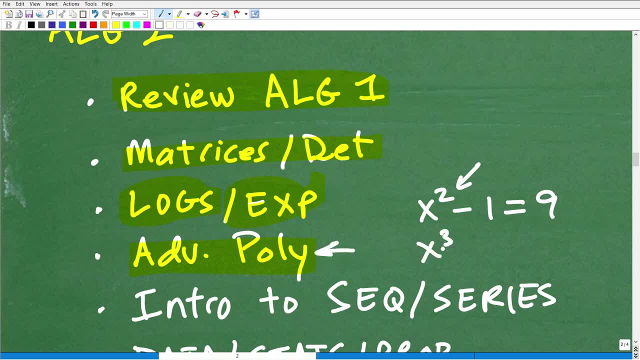 In Algebra two advanced polynomial equations you start looking at like third or fourth or fifth degree polynomials. So you start looking at like third or fourth or fifth degree polynomials And it's. this is a whole nother kind of step up And you know advanced algebra is a lot to learn. 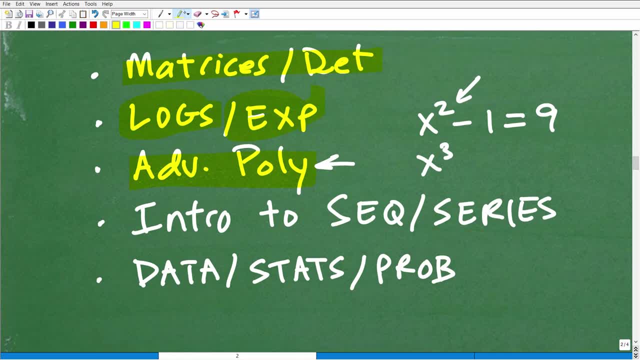 there, And a lot of these topics are going to be continued in pre calculus. you'll see this here in a second And then you're going to get into sequence and series. you may or may not, it all depends Most, I would say most Algebra. two courses will introduce you to sequence and series. 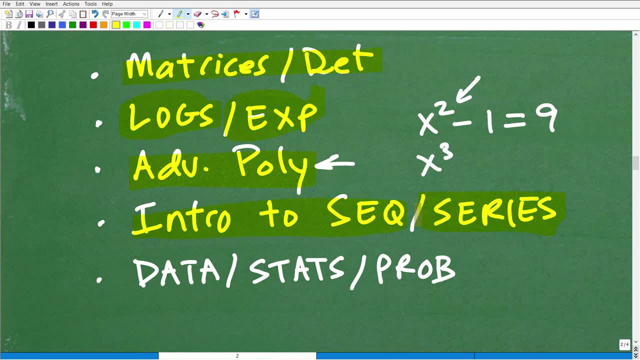 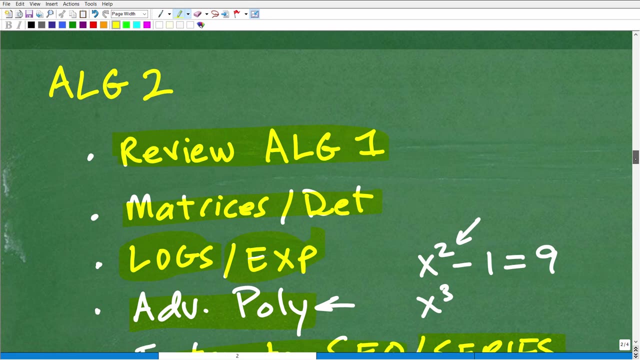 we're talking about arithmetic, geometric, infinite geometric sequence and series, And then you will continue on at a higher level to learn more about data, statistics, probability and the like. Okay, so a pretty big step up from Algebra one. okay, but if you didn't do well in 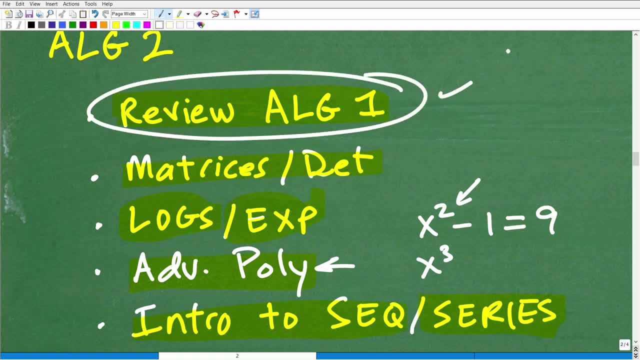 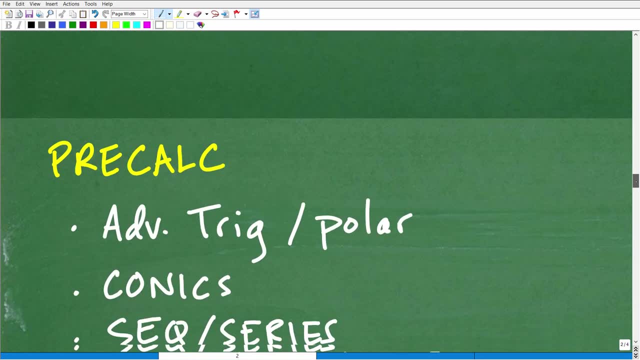 Algebra one. well, guess what? you're going to have another chance to kind of learn it again in Algebra two. all right, and then you're going to be learning obviously much more advanced stuff. Okay, so let's move on to pre calculus. So pre calculus: 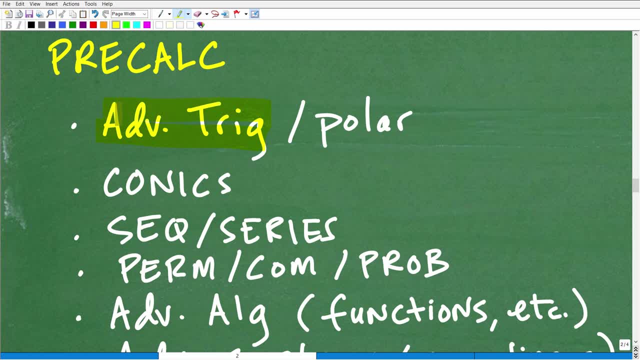 you know, is where you're going to get your advanced trigonometry. okay, And pre calculus, I would say good. third, you know one third of the actual course is trigonometry. So you're talking like three or four chapters of trigonometry, tons of different trigonometric concepts. 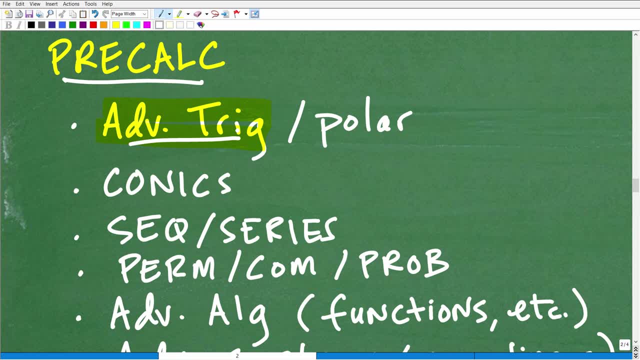 trigonometric functions, trigonometric identities, polar equations, polar coordinates. this is a big, big deal. Okay, you're definitely going to need this for calculus- Another topic they learn in pre calculus And sometimes you can find these in Algebra. two courses: 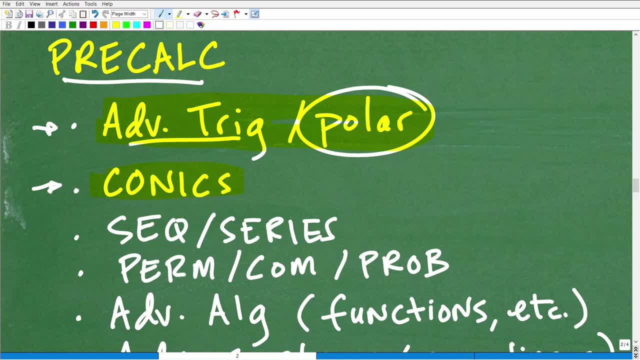 like Algebra, two trigonometry. So there is some kind of, you know, overlap, all dependent on your course. But another concept that you're going to get is what we call conic sections, So these would have to deal with shapes like circles, ellipses, hyperbolas. 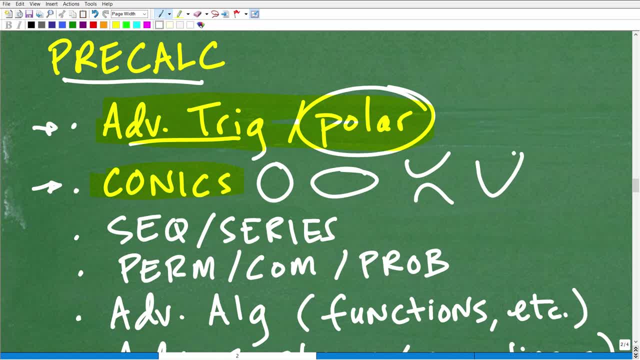 even parabolas, right? You're saying, oh, I studied parabolas and Algebra one. Well, not at this level. it's much more advanced. so that's conic sections, really, really important stuff, and you're definitely going to get into more sequence and series. okay, things like the binomial theorem and you know. 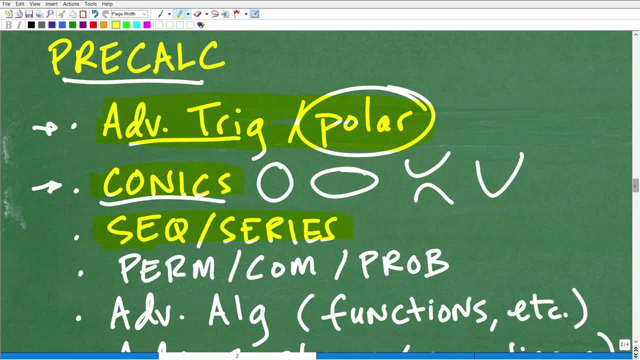 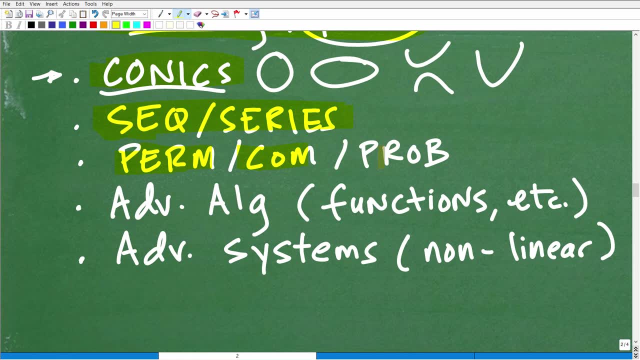 this is a really important topic to understand for calculus and then some other other things that you're going to see, and i'm just kind of breaking this out: uh, you know permutations, combinations, prob, more probability. you know, uh, solving, counting, uh problems. uh, this is important, okay, all it's all important, but uh, again, you might have seen some of this uh in your respective uh. 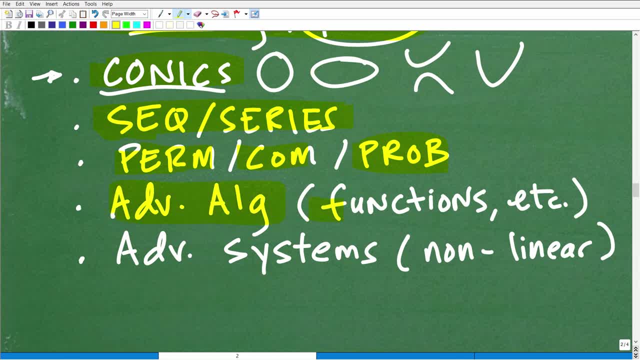 you know algebra two courses and then more advanced algebra, right like uh. you know a bigger or more intense study of functions, um, even functions, odd functions. you know analyzing domain range, etc. all this stuff you need to know to be successful in algebra and i'm not. i'm leaving stuff out here. 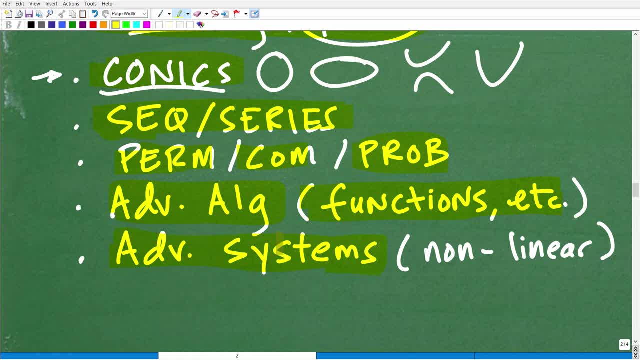 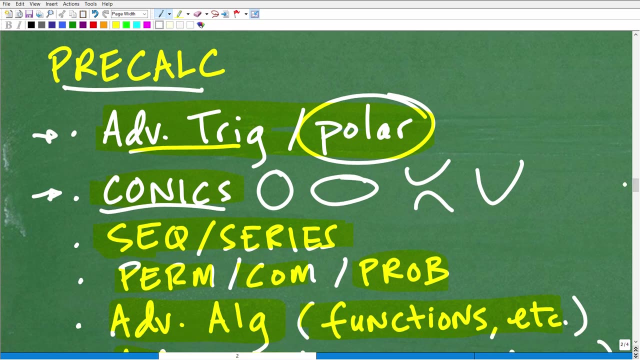 i'm just kind of highlighting some big picture stuff and then like advanced systems, all right, so these would be like non-linear systems or systems in three or four variables. so how do you deal with those? so again, i'm not including everything, i'm just trying to give you a sense of the kind of 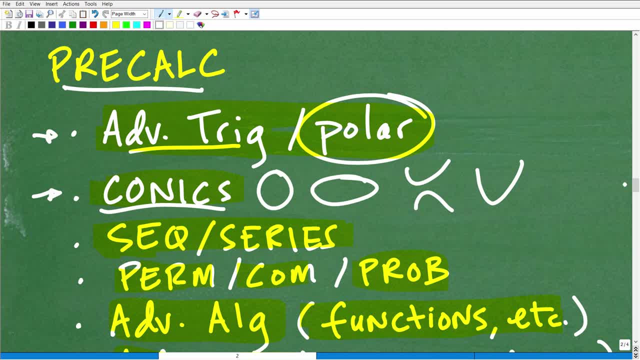 continuity between these courses. okay, so if you're thinking, boy, you want to- uh, you know, get the calculus, well, you're going to have to do a lot of things, but i'm just trying to give you a sense: have to know all this stuff. right, it's all, it's. everything kind of builds upon itself and you're. 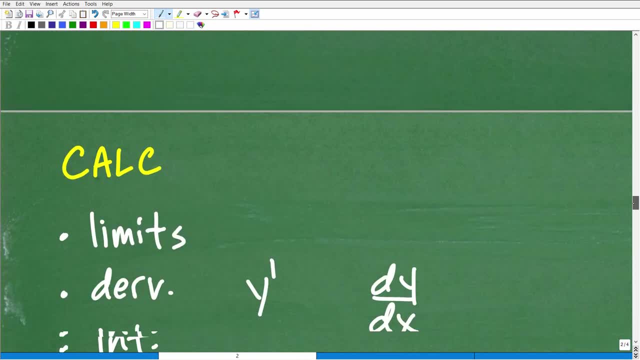 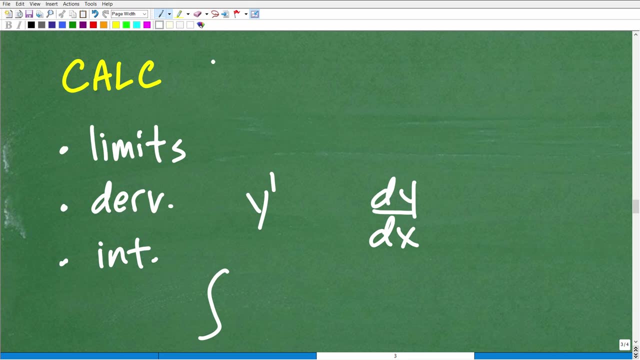 going to need it in calculus. so let's take a real, real, fast look at a typical first semester of calculus. calculus has broken up in all kinds of different ways. you have calc one, you can have calc two, you can have calc three. all depends on how your college- or whatnot- might teach it. 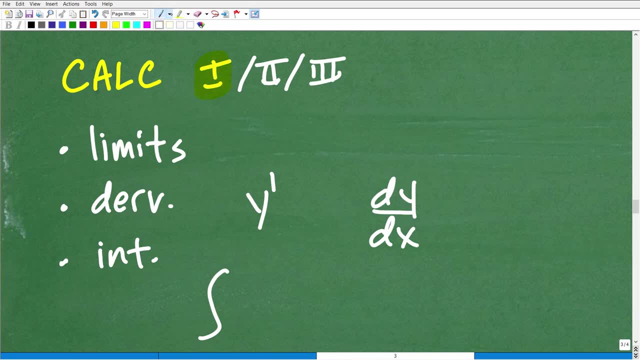 but most people who might need to just take a basic calculus course. let's say, if you're a business major, you don't have to go beyond that. so there's, you know, the more advanced levels of calculus, or like multi-level or multi-variable calculus. you know, these are for folks that are going to. 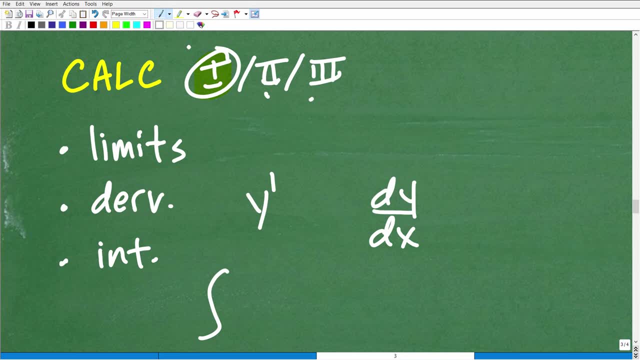 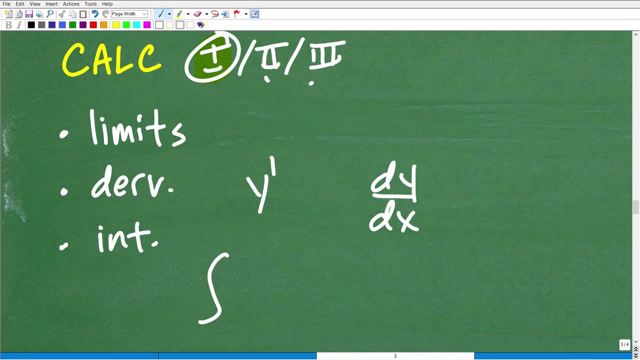 go on to become engineers etc. but you know there is a lot of people again have to take just a basic one semester of calculus, okay. so what are some of the main ideas there? well, you know, i'm just kind of highlighting again some of the things. first thing is like limits, okay. so it's like 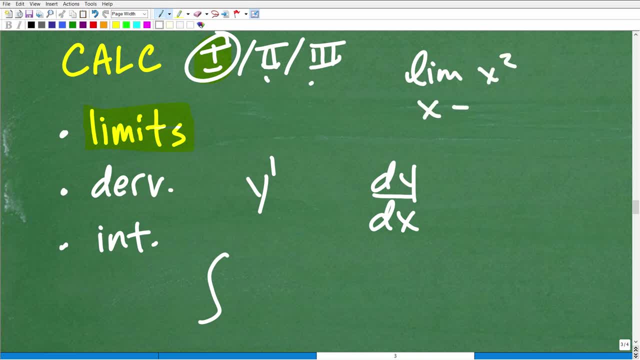 you know, limit of functions where things go to infinity. you're kind of studying the behavior of what happens when a number approaches infinity. this is a really big idea to understand. the next topic, okay in calculus, which is derivatives, and derivatives are extremely important. derivatives are is basically what makes calculus calculus it's. you know it's such a cool concept when you 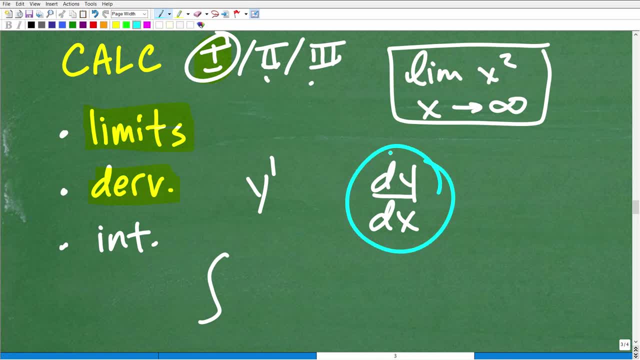 really get it. but it has to deal with rate of change, finding tangent lines and all the kind of stuff and, uh, you know, you first have to understand the concept of limits and before all that you need to have strong, strong algebra and advanced algebra skills and trigonometry skills. 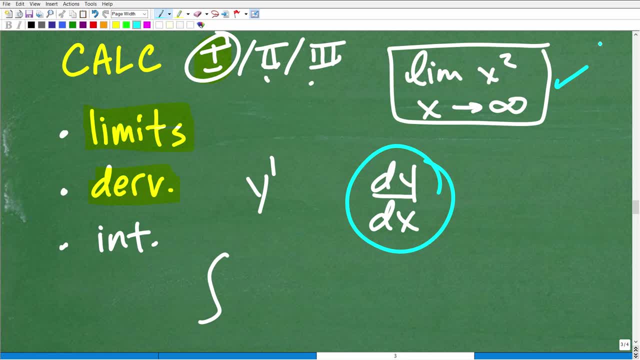 okay, because you'll be. you're going to be using all that in this course, okay. so this is just some of the basic notation that you'll see when you're working with derivatives, and then the other half of an um, a typical calculus course, you'll get into integration. it's just a little crazy long symbol. 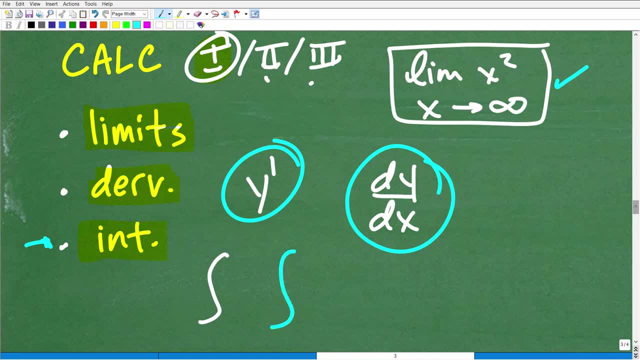 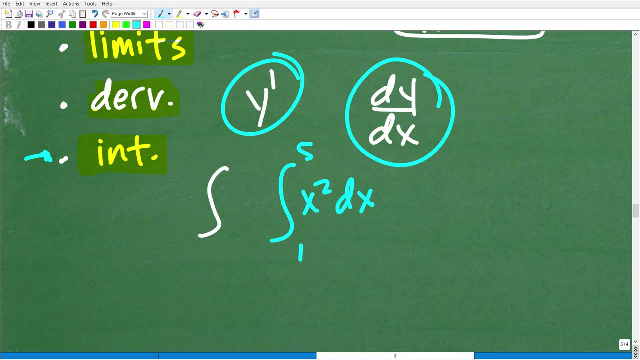 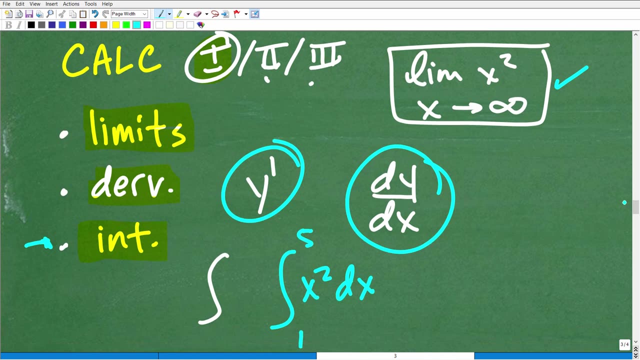 like this. it's called like an elongated s and then it has to deal with finding the area of curves: area and volumes of curves. it looks something like this. i'm just kind of making something up. so you know this is calculus. but calculus is such an awesome topic because it solves problems that 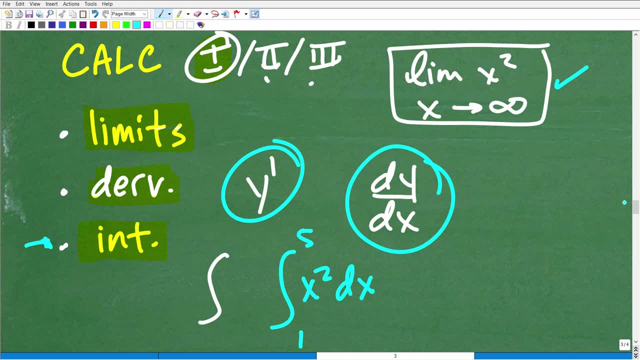 we're unable to solve, uh in with, just, you know, basic geometry and algebra. okay, you need a new mathematics that uh really kind of looks at rate of change and everything else like this. but you know, for those of you out there that are thinking about taking calculus, you could be. 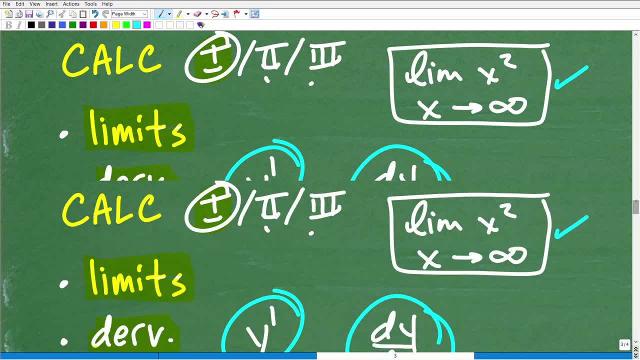 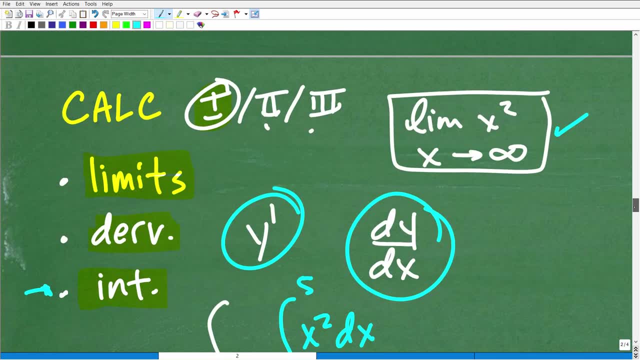 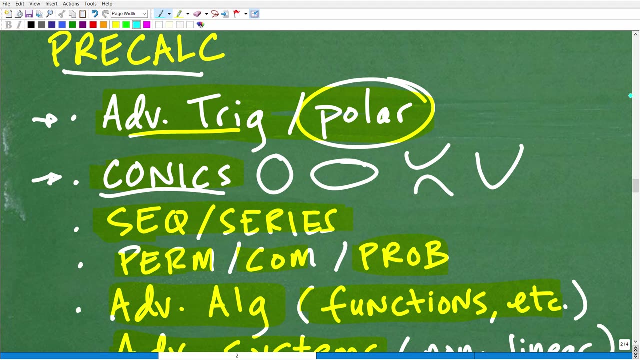 successful in them. all right, but you definitely have to have done pretty well, not perfect. you don't have to have totally 100 aced pre-calculus to be successful in calculus, but it will definitely help, right, if you didn't do too strong in pre-calculus, suppose you know. you know you've. 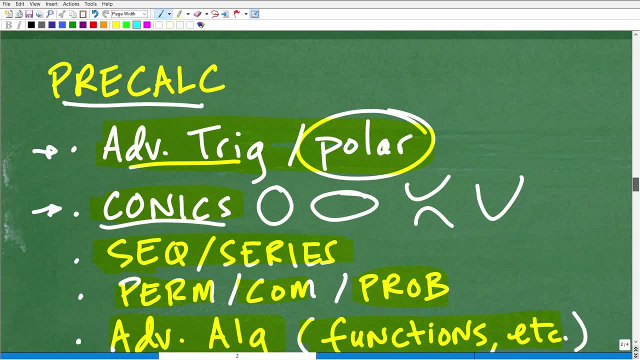 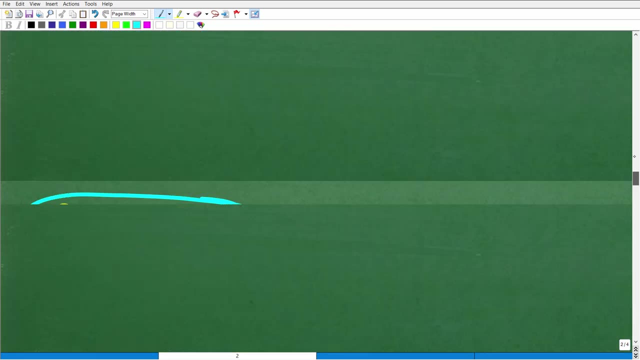 got like a, c or c plus and you know you have to take calculus for your- uh, your math class, okay, or your, your major in college or whatnot. you definitely want to do some review before you get into that calculus course, okay. so you know, brush up on your math before you take calculus. but anyways,